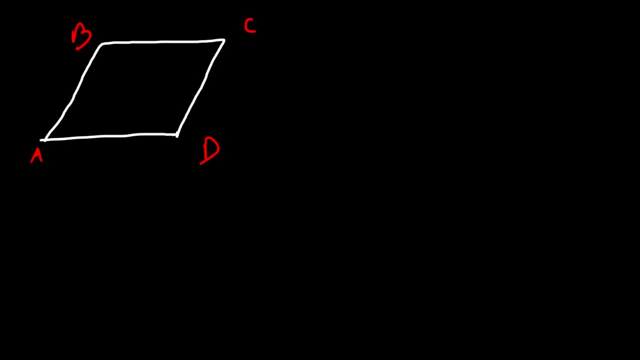 CD are congruent, then it's a parallelogram. Next, if you can show that a pair of sides are both parallel and congruent, it's a parallelogram. Now, the fourth way is to show that opposite angles are congruent. So if you can show 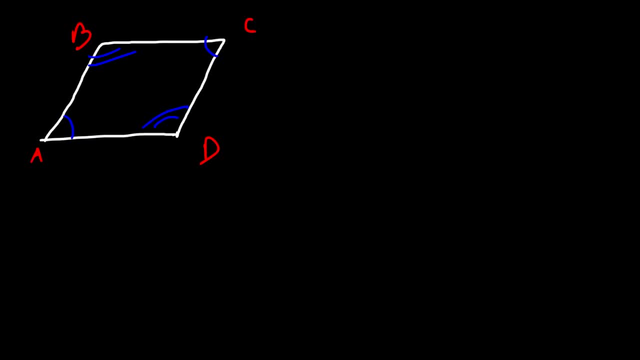 that angle B is congruent to angle D and angle A is congruent to angle C, then it's a parallelogram. Now another way is to show that the diagonals bisect each other. So let's call this E. So if you could show that, let's say, AE is congruent to EC and 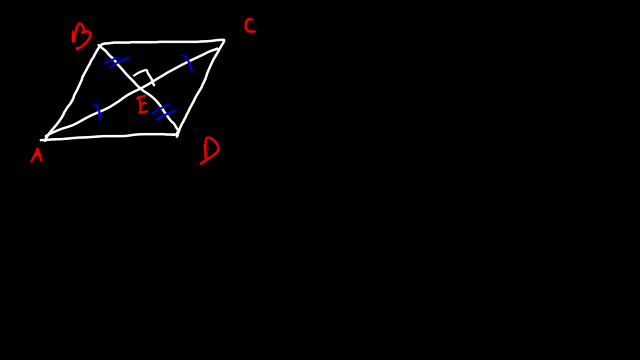 BE is congruent to ED, then it's a parallelogram. So let's try an example. Let's say this is A, B, C and D and we have a line A diagonal that connects A and C together. Now in this problem you're. 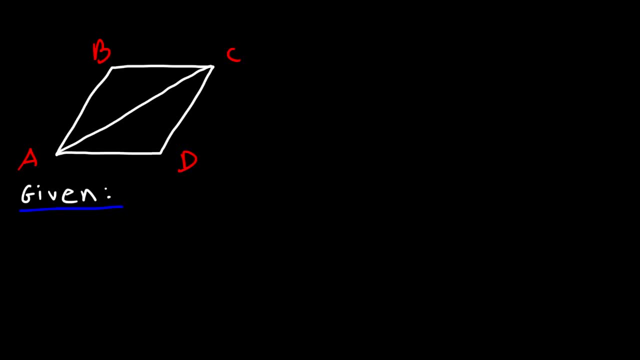 given the following information. So let's say that AB is congruent to DC and also let's say that angle BAC is congruent to angle DC, D, C, A. Your task is to prove that A, B, C, D is a. 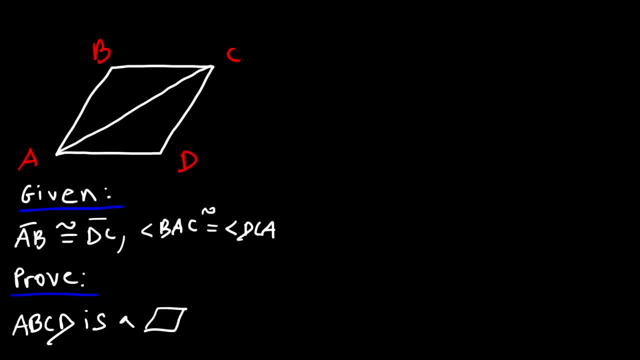 parallelogram. So let's begin. Let' s use a 2 column proof to work this out. So statements and reasons. So the first thing we should should write is the given statements. So we're given that AB is congruent to DC and the reason. 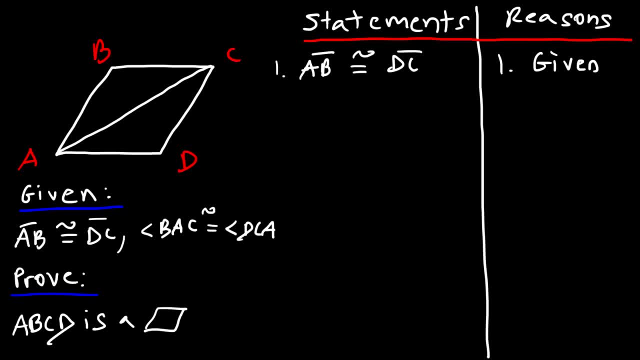 is that it's given, and so let's mark that on the graph. So this is AB and that's congruent to DC. Now, the second thing that we're given is the angles. So we know that angle BAC is congruent to DCA. So this is BAC and this is DCA. So those two are congruent and that's. 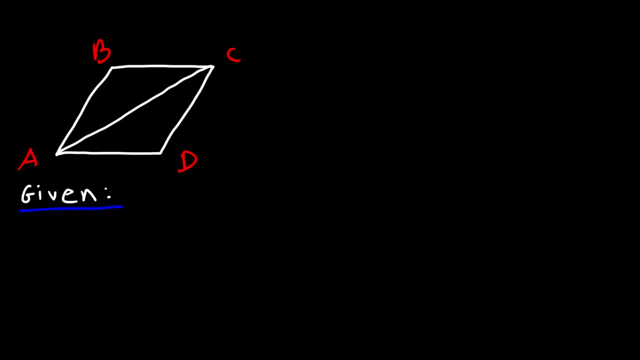 given the following information. So let's say that AB is congruent to DC and also let's say that angle BAC is congruent to angle DC. Your task is to prove that ABCD is a parallelogram. So let's begin. Let's use a two-column proof. 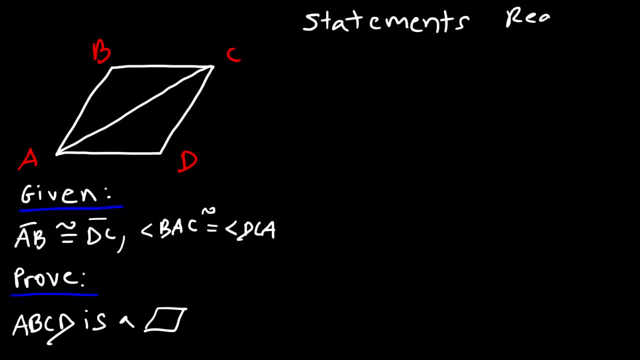 to work this out. So statements and reasons. Let's begin up with this should write is the given statements. so we're given that AB is congruent to DC, and the reason is that it's given and so let's mark that on the graph. so this is. 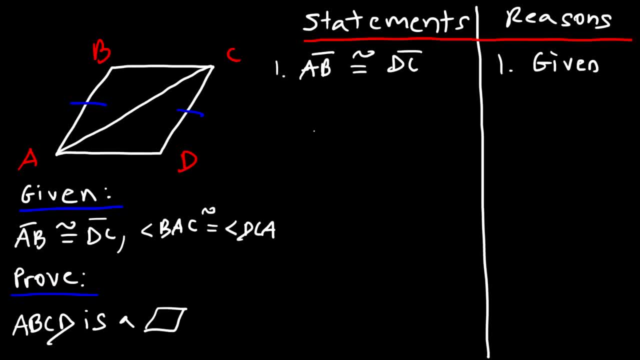 a, B, and that's congruent to DC. now the second thing that we're given is the angles. so we know that angle BAC is congruent to DCA. so this is BAC and this is DCA. so those two are congruent and that's given. now what do we need to do? 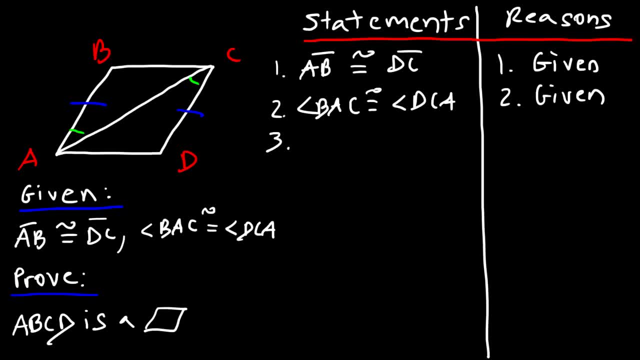 from here? where should we go? what's our next step? if we can prove the two triangles are congruent- that is triangle ABC and you CDA- then we could prove that the corresponding parts are congruent. so notice that we can use the reflexive property max so we can say that AC is 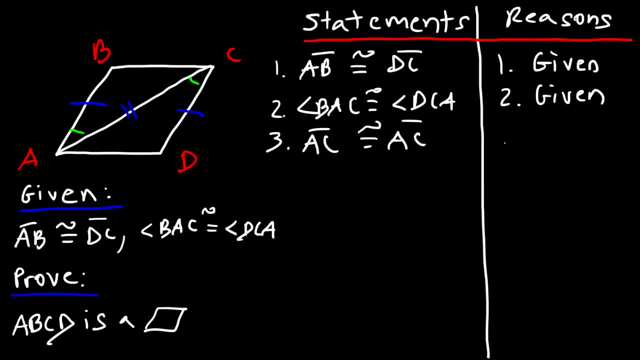 congruent to AC. it's the common side of both angles, I mean both triangles, and this is due to the reflexive property. and then number four, we can now say that triangle ABC is congruent to triangle C, DA. now what's the reason for this? why can we say this? 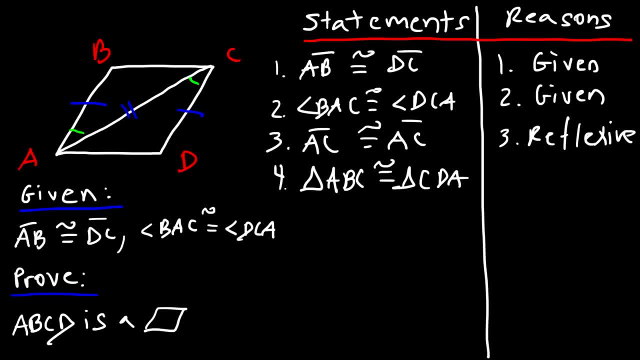 it's based on side angle side, and so that's the partial that we're using to prove that those two triangles are congruent, and we've used statements 1, 2 and 3 to show that that that partially applies. so now that the two triangles are congruent, we could 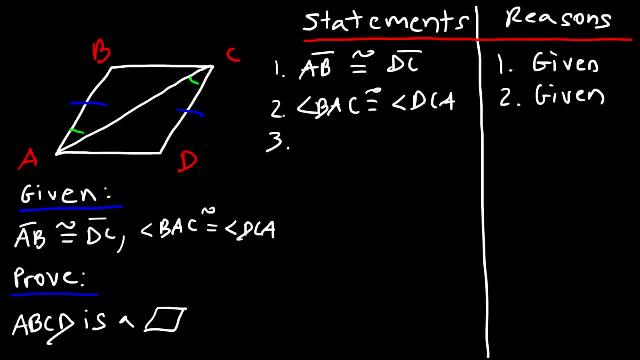 given. Now, what do we need to do from here? Where should we go? What's our next step? If we can prove the two triangles are congruent, that is, triangle ABC and CDA, then we could prove that the corresponding parts are congruent. 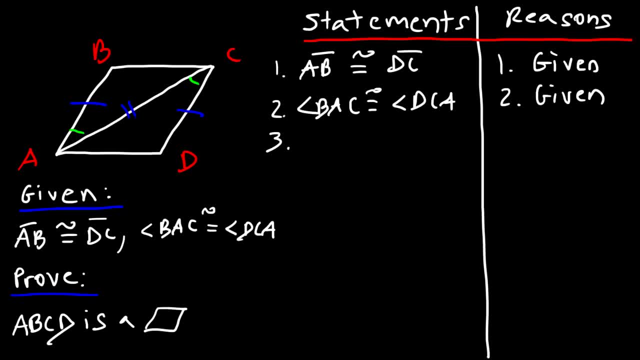 So notice that we can use the reflexive property next, So we can say that AC is congruent to AC. It's the common side of both angles, I mean both triangles, And this is due to the reflexive property. And then, number four, we can now say that triangle ABC is congruent. 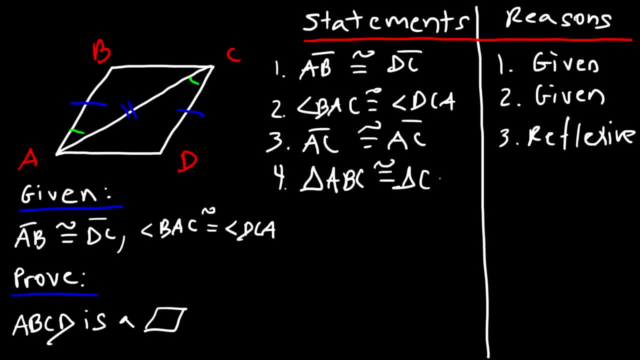 to triangle CDA. Now, what's the reason for this? Why can we say this? It's based on side angle side, And so that's the populate we're using to prove that those two triangles are congruent, And we've used statements 1, 2, and 3 to show that that populate applies. So, now that the 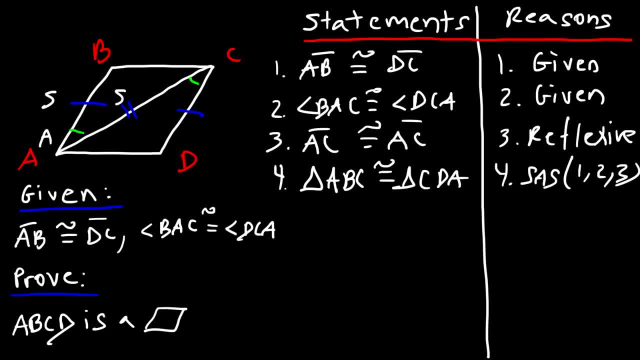 two triangles are congruent. we can say that triangle ABC is congruent, So that's the common side of the angle. triangles are congruent. we could say that BC is congruent to AD And the reason for this is CPCTC. Corresponding parts of congruent triangles are congruent. 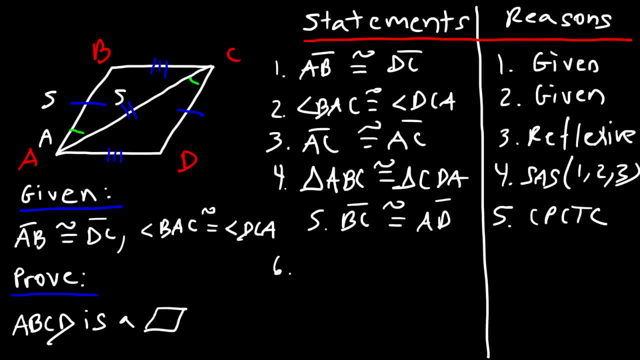 Now, in step six, we can make our final statement. We could say that ABCD is a parallelogram And the reason, definition of a parallelogram And, as we could see, if the opposite sides of a parallelogram are congruent, then the figure is a parallelogram. 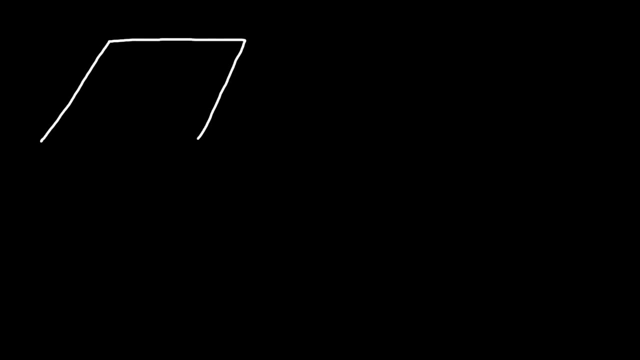 Now let's work on another example. So we're going to have a similar figure, but this time we're going to use two diagonals as opposed to one, And in this problem we're given the following information: So let's say that E is the midpoint of AC. 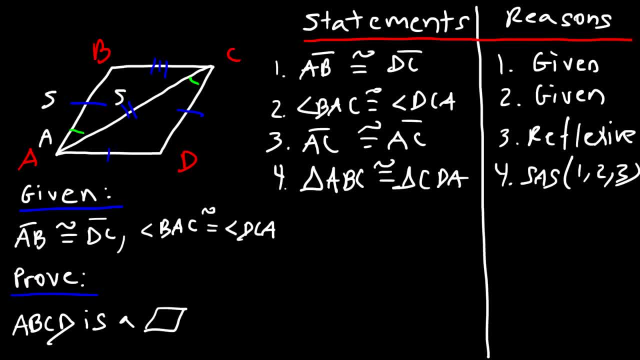 say that BC is congruent to ad and the reason for this is CP, CTC, corresponding parts of congruent triangles are congruent. now, in step six, we can make an final statement. we could say that ABCD is a parallelogram and the reason: definition of a parallelogram and, as we could see, if the opposite sides of 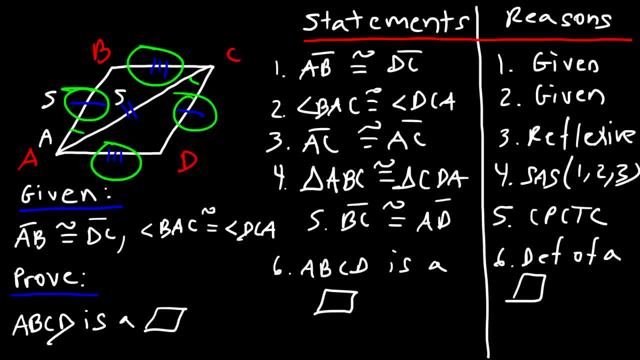 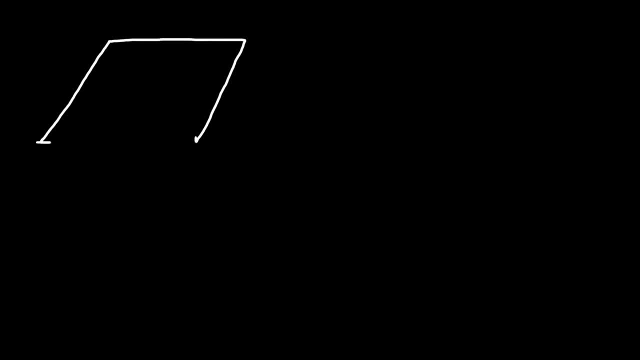 the parallelogram are congruent, then the figure is a parallelogram. now let's work on another example. so we're going to have figure, but this time we're going to use two diagonals as opposed to one, and in this problem we're given the following information: so let's say that E is the 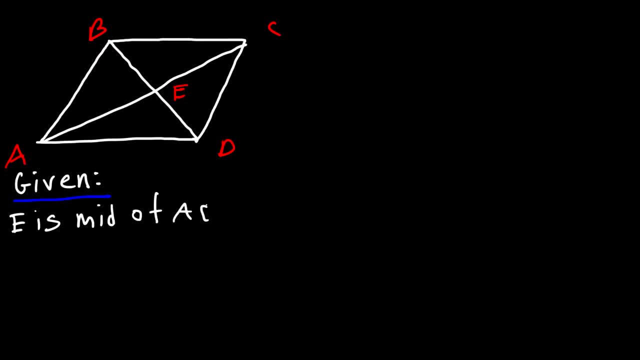 midpoint of AC, and let's also say that angle EAD is congruent to angle ECB. our goal in this problem is to prove that ABCD is a parallelogram. so, just like before, we're going to use a two column proof statements and the reasons for those statements. so if you want to pause the video and try this, 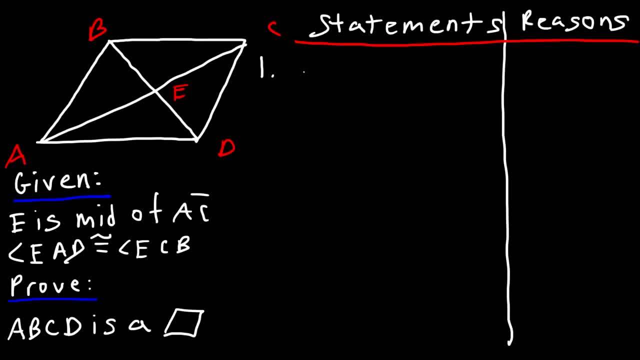 problem. so let's begin with the given statement. E is the midpoint of AC, and so that's given. so what can we conclude from this given statement? if E is the midpoint of AC, that means that AE has to be congruent to EC. so let's write. 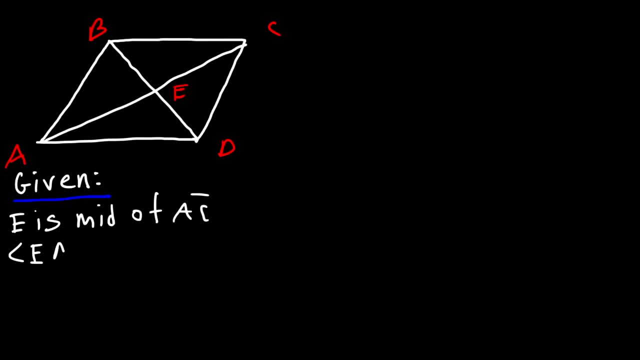 And let's also say that angle EAD is congruent to AC. And let's also say that angle EAD is congruent to AC, And let's also say that angle EAD is congruent to angle ECB. Our goal in this problem is to prove that ABCD is a parallelogram. 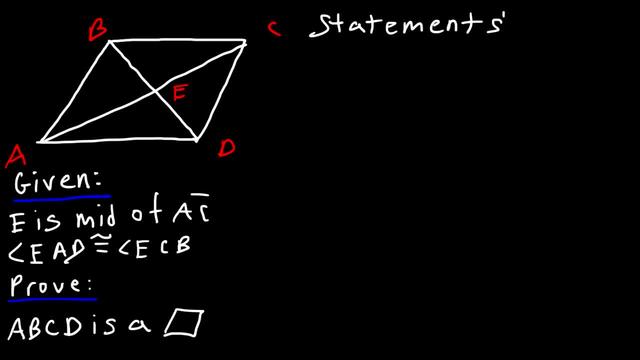 So, just like before, we're going to use a two-column proof Statements and reasons for those statements. So if you want to pause this video and try this problem, So let's begin with the given statement. E is the midpoint of AC. 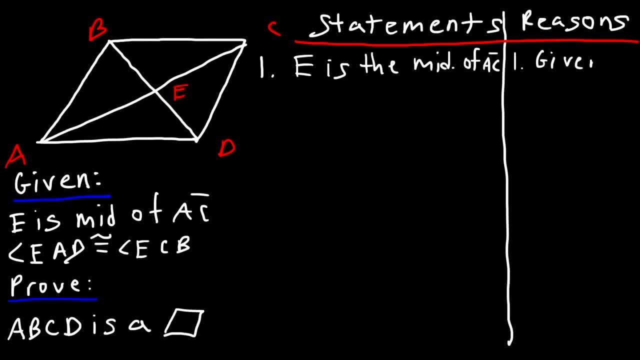 And so that's given. So what can we conclude from this given statement? If E is the midpoint of AC, that means that AE has to be congruent to EC. So let's write that. So AE is congruent to EC. and the reason for this definition of a midpoint. 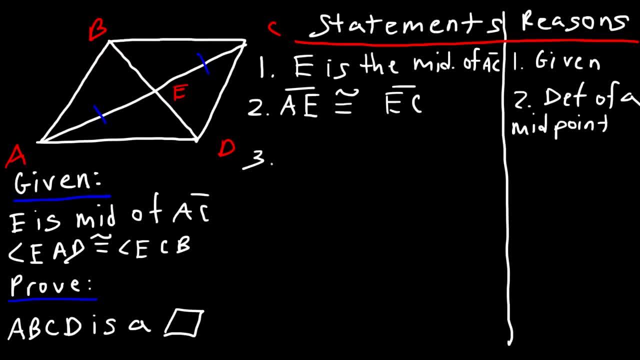 Now let's move on to number three. What else can we say? Notice that these two angles are congruent. They form vertical angles. So we could say that AED is congruent to angle CED. So this is AED and this is CED. 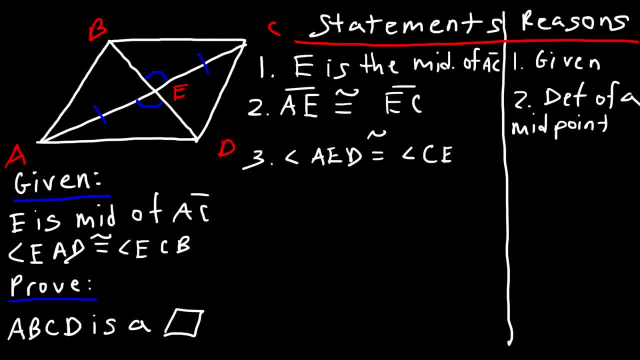 I mean, that's supposed to be CEB rather, So let's just put a B here. And the reason for that is that vertical angles are congruent. Now, because I'm running out of space, I'm going to put VAT V-A-T vertical angle theorem. 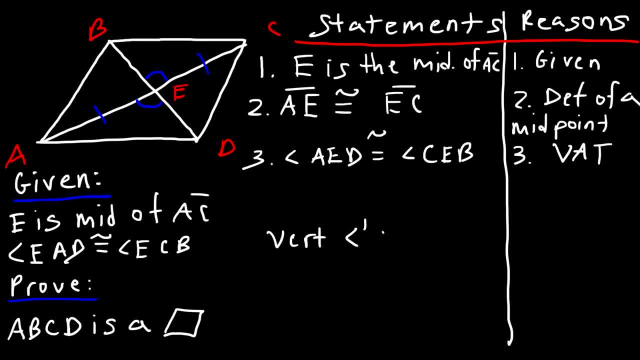 But you can also write it this way: Vertical angles are congruent if you want to. It's just I didn't put too much space in that column, so I'm going to have to be creative with the ways I'm writing for the reasons in that column. 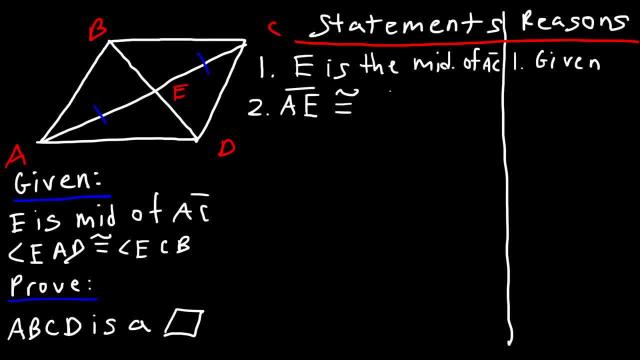 that. so AE is congruent to EC, and the reason for this definition of a midpoint. now let's move on to number three. what else we say? notice that these two angles are congruent. they form vertical angles. so we could say that AED is congruent to angle CED. so this is AED and this is. 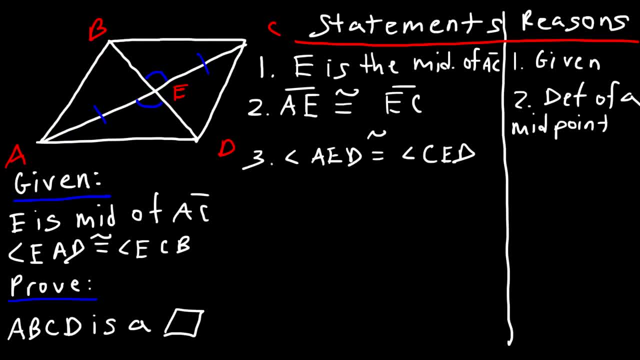 CED- I mean, that's supposed to be CEB, rather, so let's put it be here- and the reason for that is that vertical angles are congruent. now, because I'm run out of space, I'm gonna put VAT vertical angle theorem, but you can also write it this way: vertical angles are congruent. 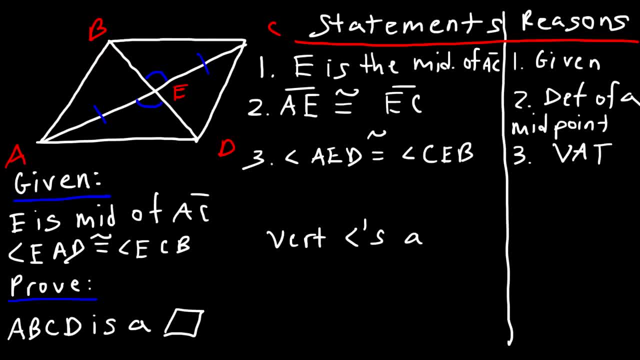 if you want to. it just I didn't put too much space in that column, so I'm gonna have to be creative with the ways I'm writing, for the reasons in that column I Now there's something else that we could write too, and that is the second given statement. 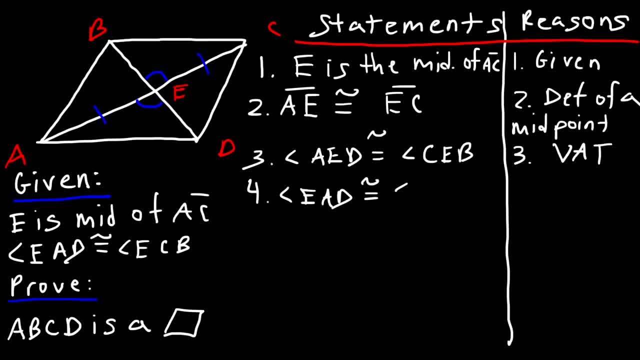 So angle EAD is congruent to angle ECB. So this is angle EAD and this is ECB. So therefore, this angle is congruent to that angle And so let's write that. So the reason for this it's given. Now notice that we can prove that this triangle is now congruent to this triangle. 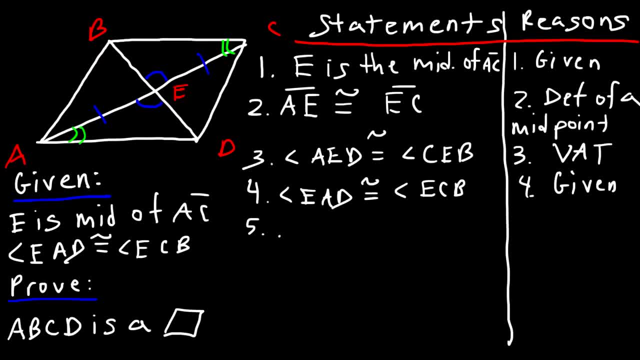 So we can make the statement that triangle AED is congruent to triangle CEB, And this is based on the angle side Side angle postulate And so far we've used statements 2,, 3, and 4 to prove it. 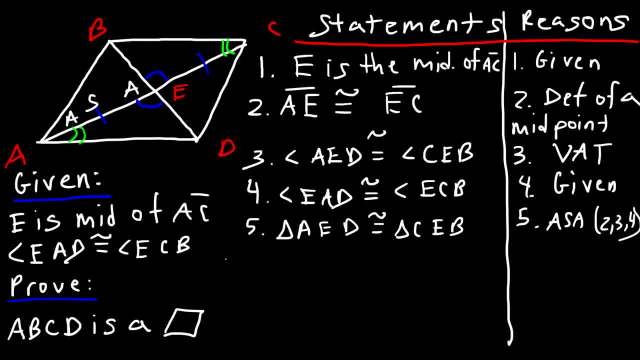 So I'm going to write 2,, 3, 4.. So now, if those two triangles are congruent, then the corresponding parts of those triangles are congruent as well. So we could say that ED and BE are the same because they're parts of those two triangles. 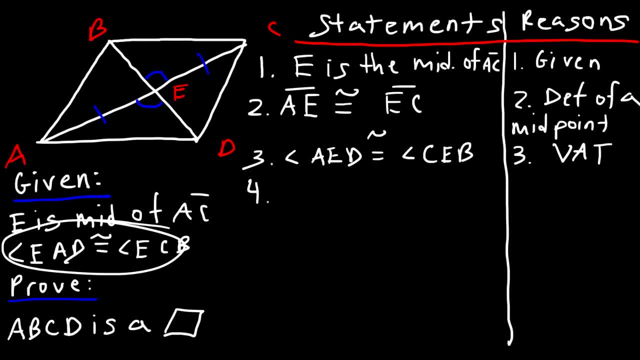 Now there's something else that we could write too, And that is the second given statement. So angle E EAD is congruent to angle ECB. So this is angle EAD and this is ECB. So therefore, this angle is congruent to that angle. 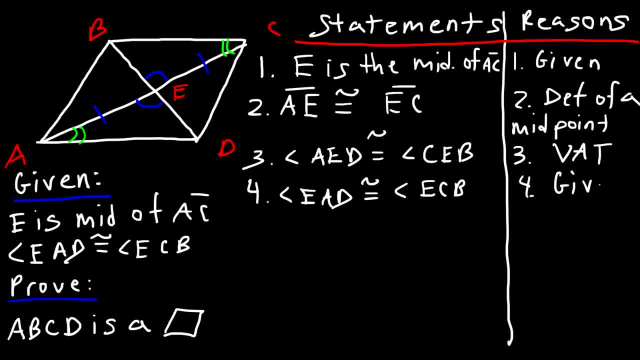 And so let's write that. So the reason for this it's given. Now notice that we can prove that this triangle is now congruent to this triangle, So we can make the statement that triangle AED is congruent to triangle CEB. 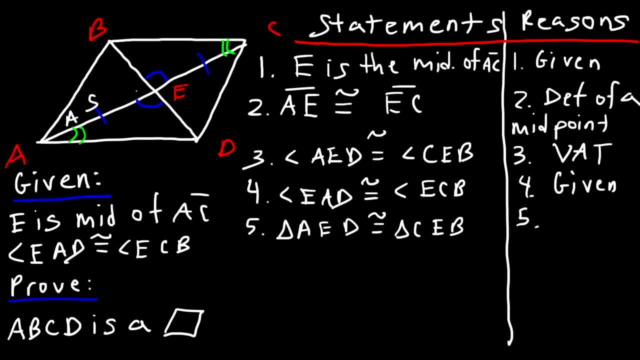 And this is based on the angle-side-angle postulate And so far we've used statements 2,, 3, and 4 to prove it. So I'm going to write that. I'm going to write 2,, 3, 4.. 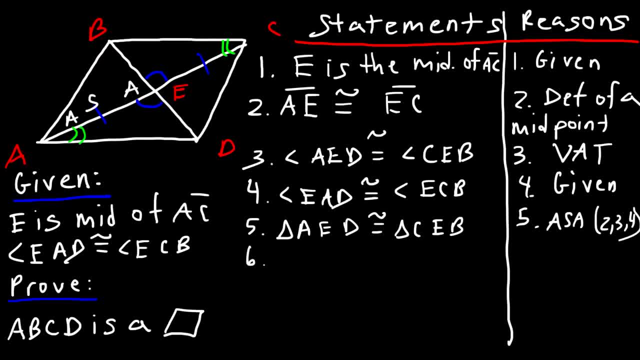 So now, if those two triangles are congruent, then the corresponding parts of those triangles are congruent as well. So we can say that ED and BE are the same because they're parts of those two triangles that we've just proven. 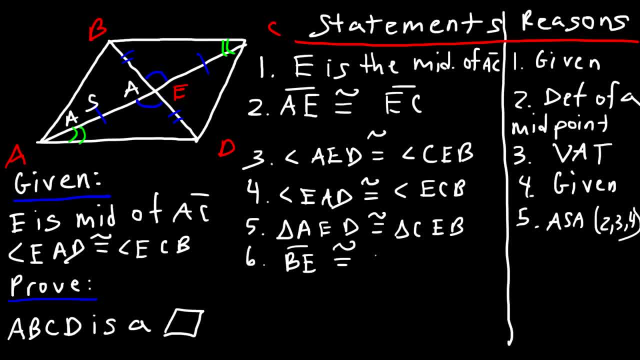 So let's say that BE is congruent to ED. So let's say that BE is congruent to ED, And the reason for this is that the corresponding parts of congruent triangles are congruent. Now notice that these two parts are congruent to each other. 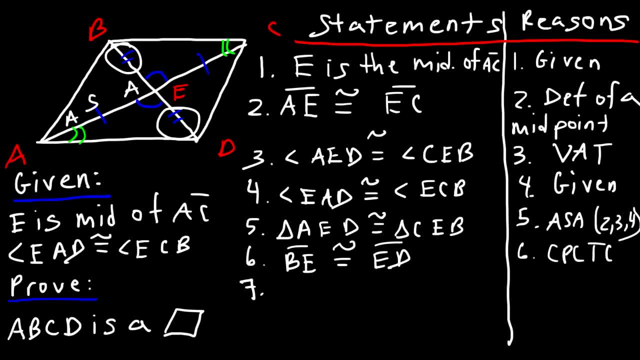 and those two parts are congruent to each other. So we could say that AC bisects BD And we could also say that BD bisects AC. And the reason: definition of a segment bisector. Now, because the two diagonals, AC and BD, bisect each other. 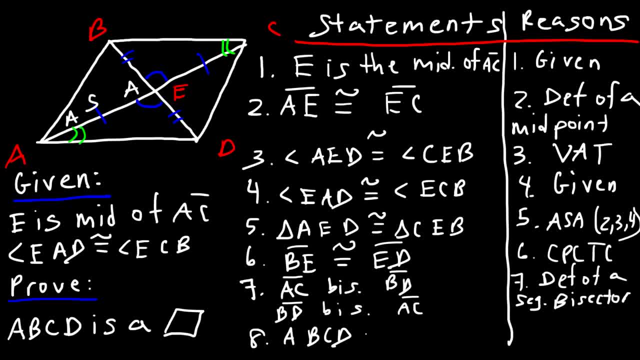 we can now make a final statement that ABCD is a parallelogram And the reason for this is the definition of a parallelogram. So if you can prove that the diagonals BD bisect each other, which we did, 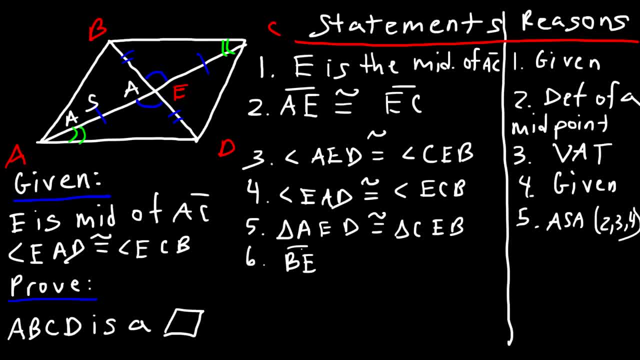 that we've just proven. Okay, So let's say that BE is congruent to ED And the reason for this? CPCTC Corresponding parts of congruent triangles are congruent. Now notice that these two parts are congruent to each other and those two parts are congruent. 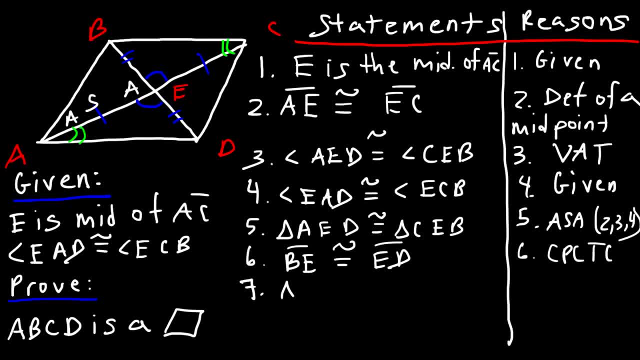 to each other. So we could say that AC bisects And we could also say that BD bisects AC. And the reason: definition of a segment bisector. Now, because the two diagonals, AC and BD, bisect each other, we can now make a final statement. 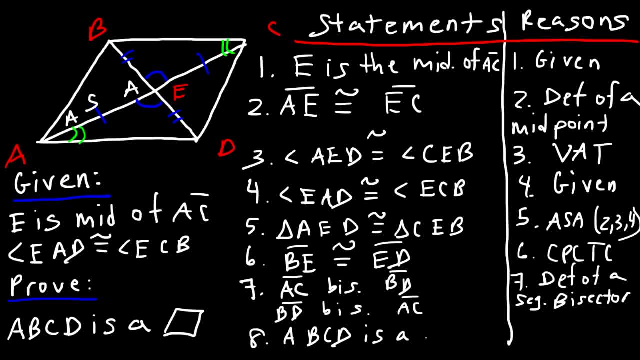 that ABCD is congruent. Okay, AC bisector is a parallelogram And the reason for this, the definition of a parallelogram. So if you can prove that the diagonals bisect each other, which we did, then that means. 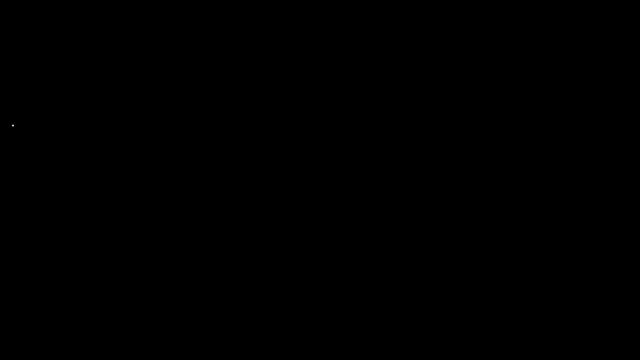 that the figure is a parallelogram. Let's work on one more example. So let's say: this is A, A, B, C and D. We're gonna call this E and F. So here's the information that we're given in this problem. 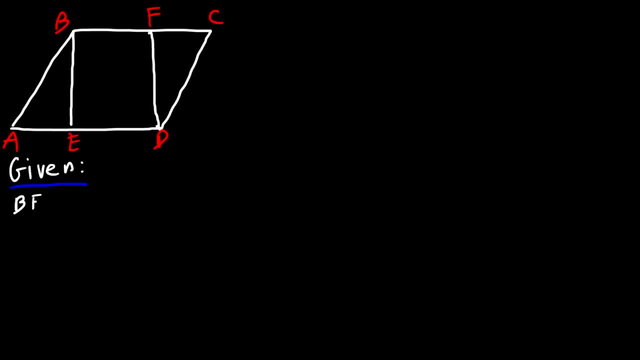 So first we're given that BEDF is a parallelogram- So that's the first thing we're given- And that angle AEB, ISIS. Now, what do we do? We multiply is congruent to angle GFD. Now, the third thing we're given is that 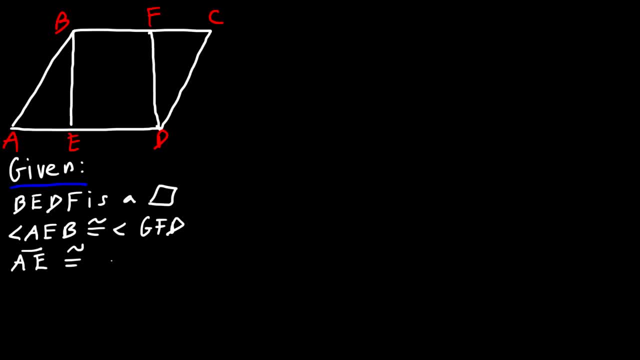 AE is congruent to FG. So with this information, let's prove that ABCD is indeed a parallelogram. So we're given a parallelogram and we're going to use it to prove that another parallelogram is indeed a parallelogram. 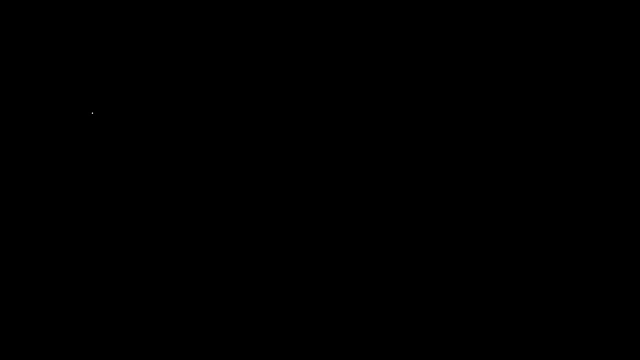 then that means that the figure is a parallelogram. Let's work on one more example. So let's say this is A, B, C and D. We're going to call this E and F. So here's the information that we're given in this problem. 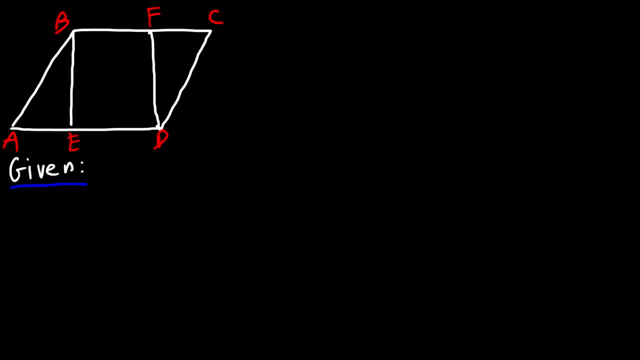 So first we're given that BEDF is a parallelogram- So that's the first thing we're given- And that angle AEB is congruent to angle GFD. Now the third thing we're given is that AE is congruent. 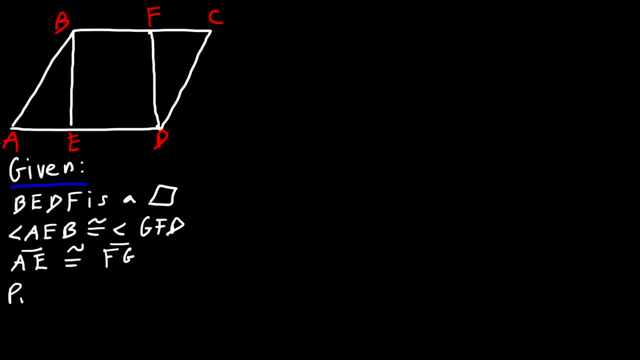 to FG. So with this information, let's prove that ABCD is indeed a parallelogram. So we're given a parallelogram and we're going to use it to prove that another parallelogram is indeed a parallelogram. 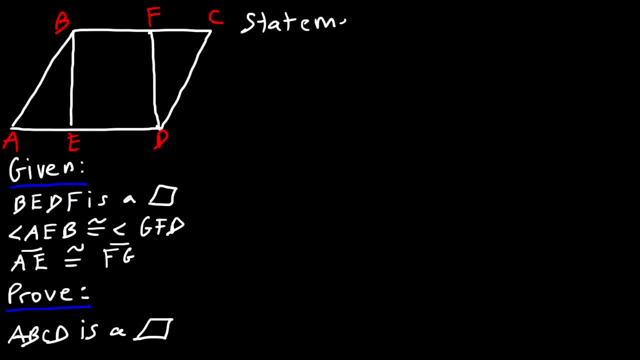 So let's use a two-column proof- Statements And reasons- And I need to fix a small mistake that I made which can have some serious consequences. So this is supposed to be CFD And this is CF- CF. 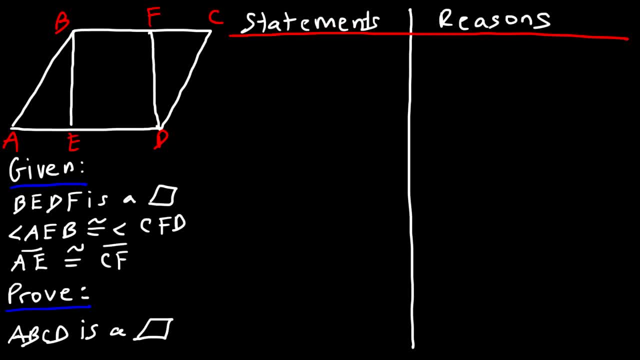 Or you could say: FCCD, now go ahead and try this problem. so let's start with number one, our first given statement. so b, e, d, f is a parallelogram, and so that's given to us now the fact that this is a parallelogram. what information can we glean from it? 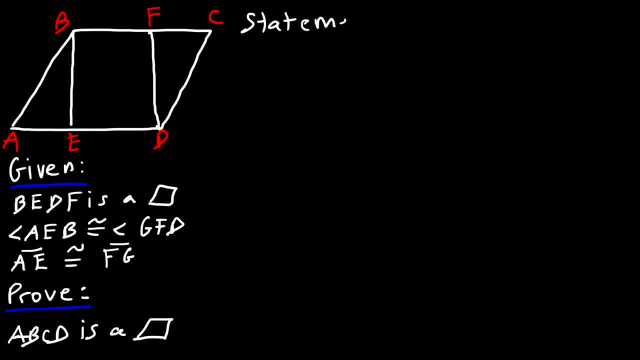 So let's use a two-column proof- Statements and reasons- And I need to fix a small mistake that I made which can have some serious consequences. So this is supposed to be CFD And this is CF, Or you could say FC. 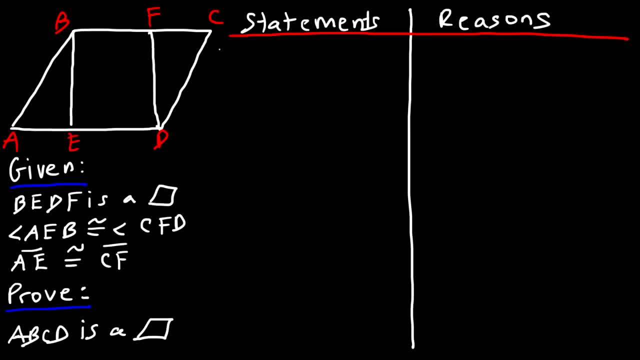 Now go ahead and try this problem. So let's start with number one, our first given statement. So BEDF is a parallelogram, And so that's given to us Now the fact that this is a parallelogram. 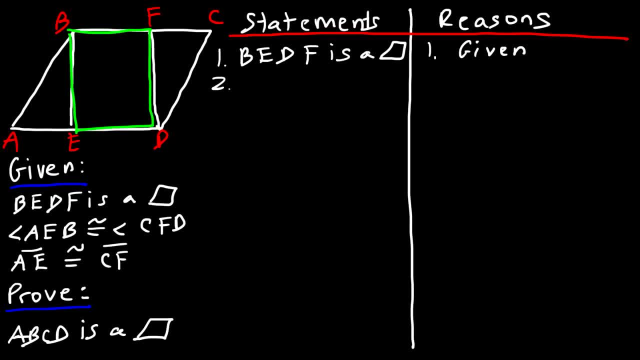 what information can we glean from it? We know that the opposite sides of a parallelogram are congruent, So BE and FD are congruent, And the reason for that is that opposite sides of a parallelogram are congruent, And the reason for that is that: 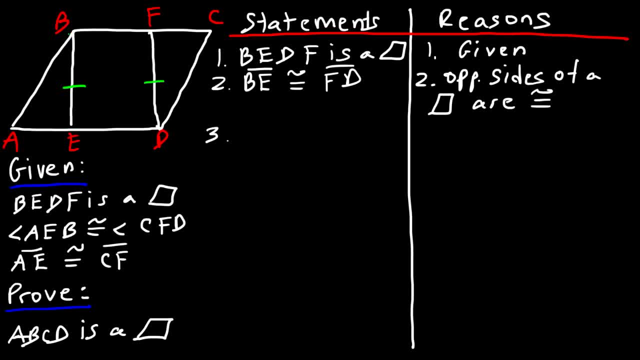 the opposite sides of a parallelogram are congruent. Now, these two are also opposite sides, So we could say that BF is congruent to ED, And so the reason for this, we could say, is the same as number two. 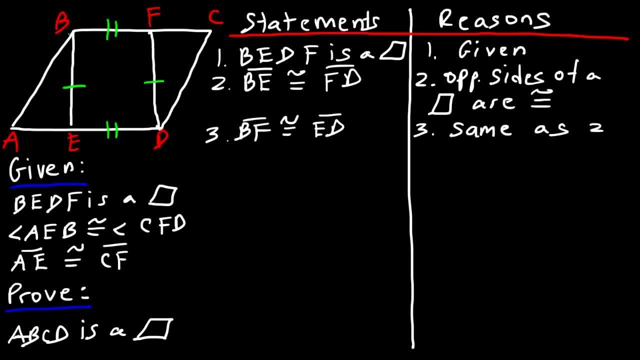 Opposite sides of a parallelogram are congruent. Now let's move on to our next given statement. that's this one. so angle AEB is congruent to angle CFD, and so that's given to us. so on, the figure here is AEB and this is CFD, so those two angles are. 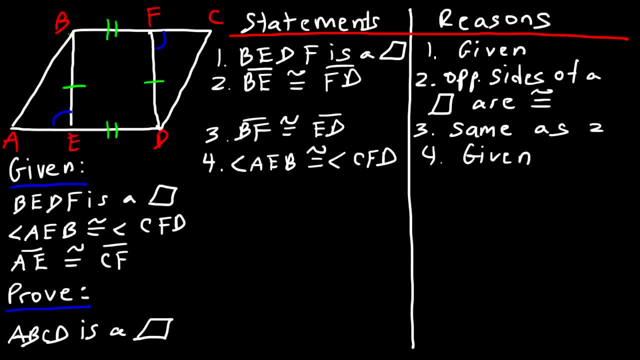 congruent. now, what else can we do? well, let's move on to our next given statement. so number five, and that's AE, is congruent to CF, and so that's given to us as well. and so this is AE, which I need to put three marks, and that's FC, or 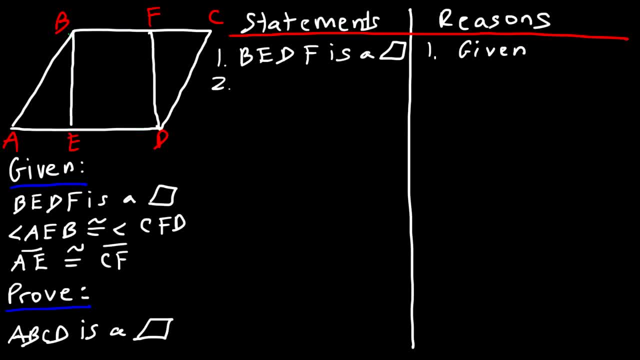 we know that the opposite sides of a parallelogram are congruent. so b, e and f- d are congruent, and the reason for that is that opposite sides of a parallelogram are congruent. now these two are also opposite sides, so we could say that b- f is congruent to 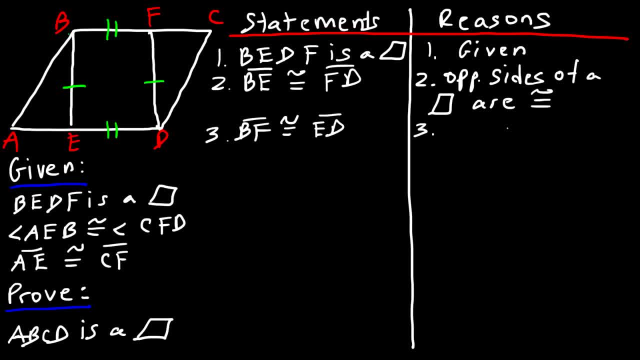 ed, and so the reason for this? we could say it's the same as number two opposite sides of a parallelogram are concrete. now let's move on to our next given statement, and that's this one. so angle is congruent to angle CFD, and so that's given to us. so, on the figure here is a. 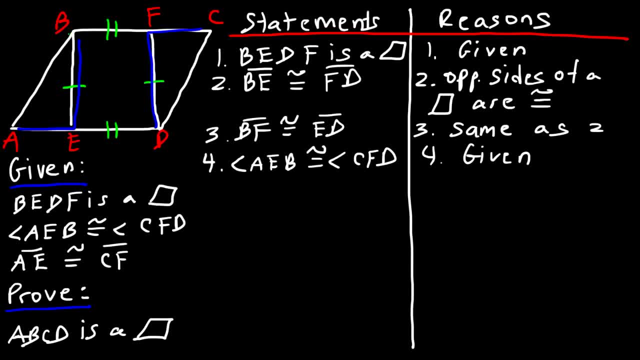 EV and this is CFD, so those two angles are congruent. now, what else can we do? well, let's move on to our next given statement. so number five, and that's a E, is congruent to CF, and so that's given to us as well, and so this is a E, which I 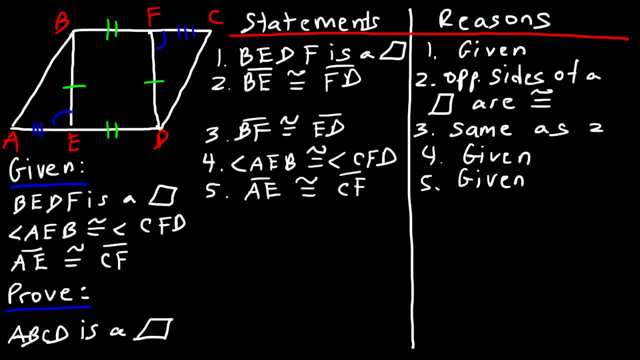 need to put three marks, and that's FC or CF. now notice that these two are congruent, and those two are congruent, so the sum must be congruent as well. so if a E is congruent to FC and if ED is congruent to BF, then their sums must be. 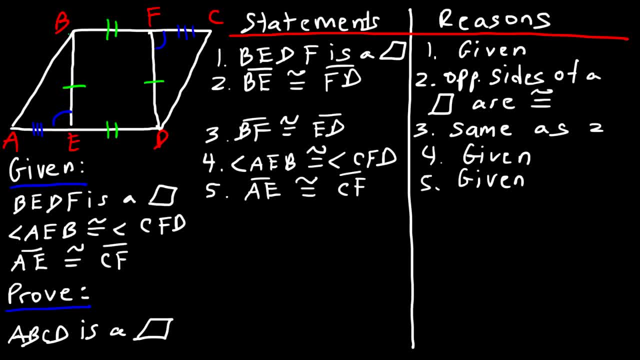 CF. now notice that these two are congruent, and those two are congruent, so the sum must be congruent as well. so if AE is congruent to FC and if ED is congruent to BF, then their sums must be congruent to each other. so AE and ED, which is AD, has to be congruent to BF and FC, which is 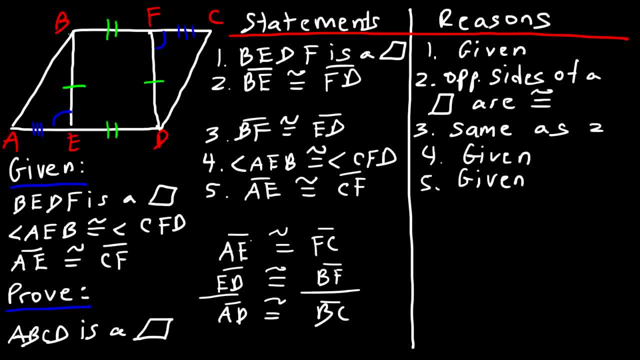 is basically BC. Now let's change our congruent statements into equality statements. So in step 6, I'm going to say that BF is equal to ED and also that AE is equal to CF, And this is going to be based on definition of congruent segments. 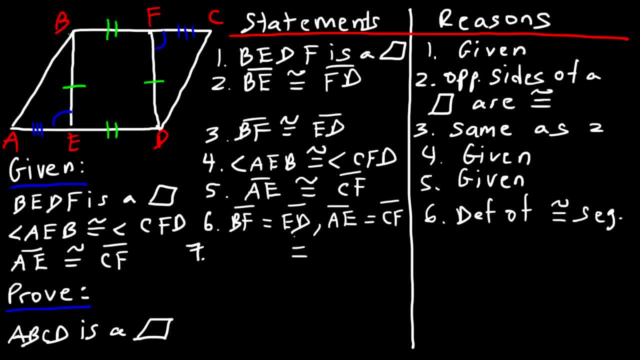 Now let's focus on this, So we can see that AE is equal to CF And CF are equal to each other. So what I'm going to do is add BF to both sides, Let's say if 5 equals 5, and then I add 3 to both sides. 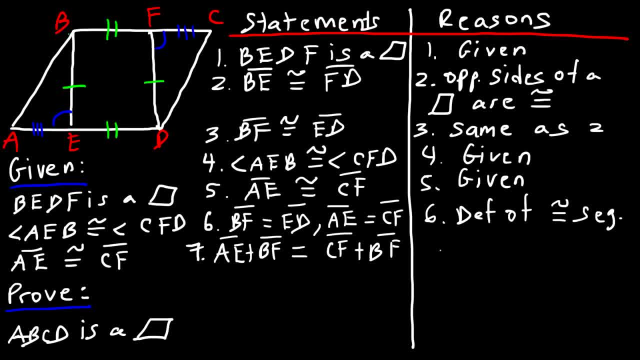 5 plus 3 equals 5 plus 3, so 8 equals 8.. So I can do that, And this is based on the addition property, The addition property of equality, And so in step 8, I'm going to replace BF. 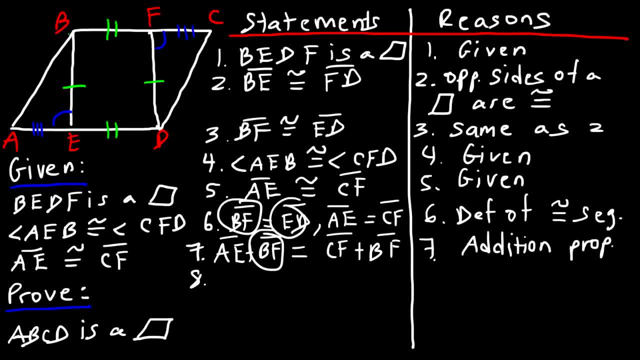 I'm going to replace BF with ED, because BF is equal to ED. So I'm going to substitute BF with ED. So I'm going to have AE plus ED and that's equal to CF plus BF. So this is based on the substitution property. 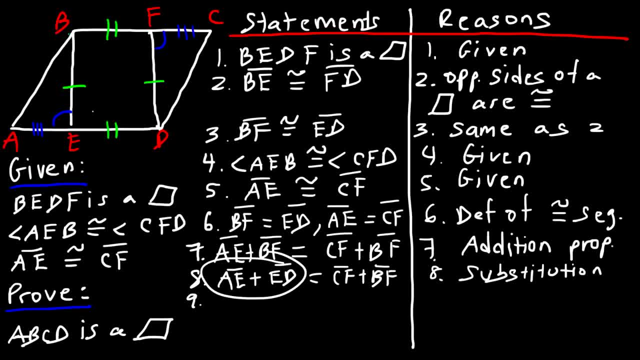 And then in step 9, notice that AE and ED they equal AD, So this is based on the substitution property. And then in step 9, notice that AE and ED they equal AD And CF and BF is equal to BC. 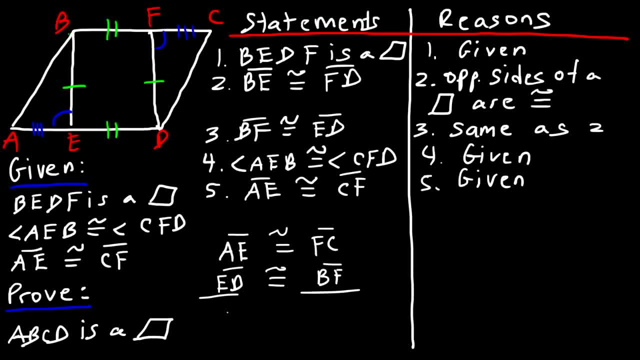 congruent to each other. so AE and ED, which is AD, has to be congruent to BF and FC, which is basically BC. now let's change our congruent statements into equality statements. so in step six, I'm going to say that BF is equal to ED and also that AE is equal to. 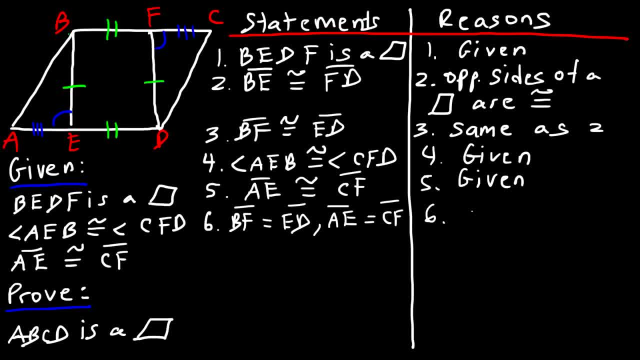 CF, and this is going to be based on definition of congruent segments. now let's focus on this so we can see that AE and CF are equal to each other. so what I'm going to do is add BF to both sides- let's say, if 5 equals 5, and then add 3 to both sides, 5 plus 3 equals 5 plus 3. so 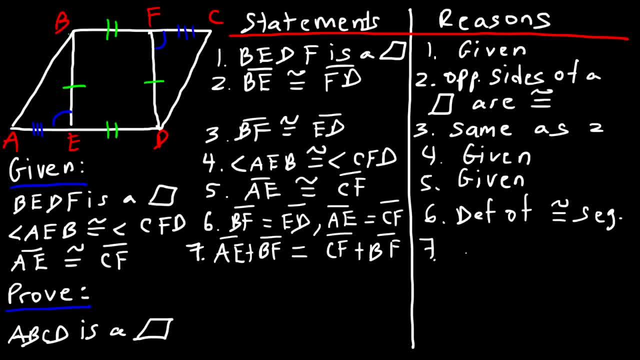 8 equals 8. so I can do that. and this is based on the addition property, the addition property of equality. and so in step 8, I'm going to replace BF with ed, because BF is equal to ed. so I'm going to substitute BF with ed. so I'm going to 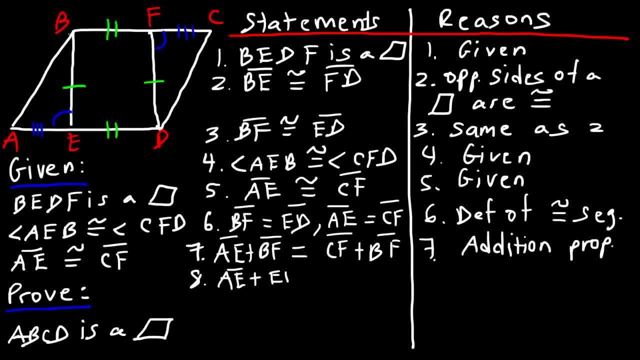 have a e plus ed and that's equal to CF plus BF. so this is based on the substitution property. and then in step 9 notice that AE and ed the equal ad, and CF and BF is equal to BC. so this is segment addition. and then in step 10 I could say that ad is now. 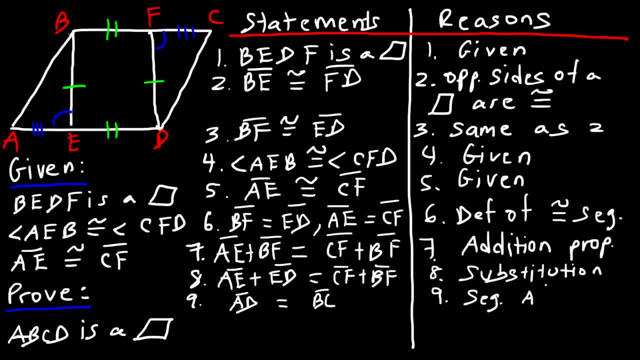 So this is segment addition. And then, in step 10, I can say that AD is now congruent to BC, And this is- This is definition of congruent segments. So now that we've shown that these two parts are congruent, we just need to show that these 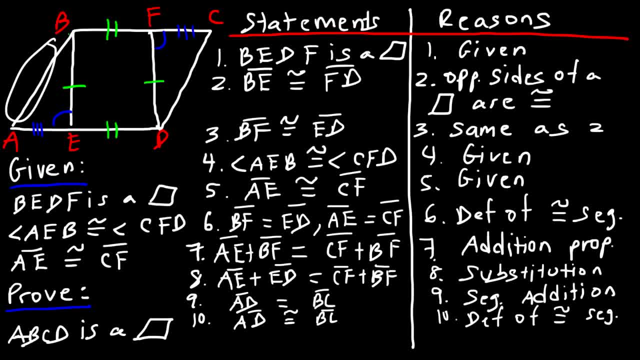 two are congruent to each other, And then we can prove that ABCD is a parallelogram. So for number 11, notice that we can prove the triangles are congruent using side angle and triangle. So let's make the statement that triangle ABE is congruent to triangle CDF. 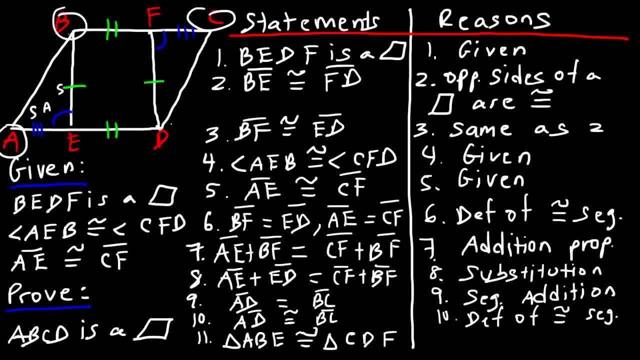 So A corresponds to C, B corresponds to D and E corresponds to F. So this is based on the SAS postulate. And then in step 10, notice that AD is now congruent to CDF. So this is based on the SAS postulate. 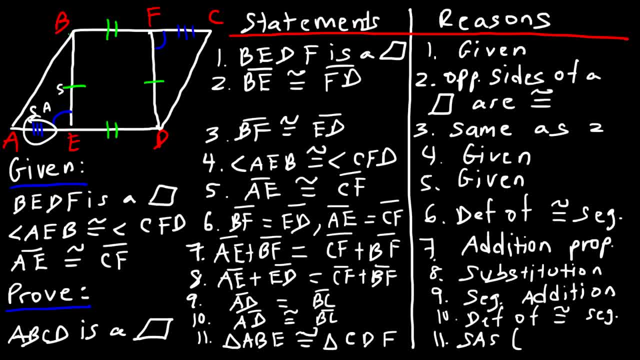 And then, in step 11, notice that AD is now congruent to CDF. So this is based on the SAS postulate, And we've used AE, which is based on statements 5.. And AEB, which is based on statements 4.. 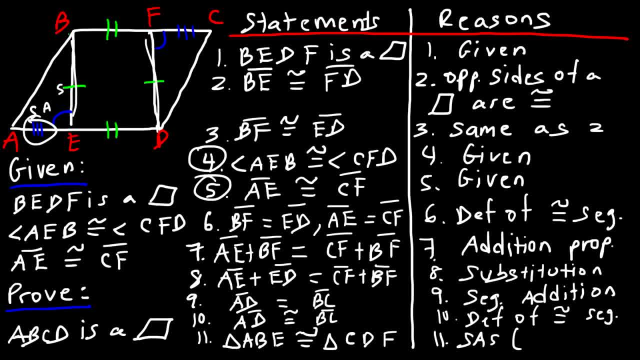 And also, BE is equal to FD, which is based on 2.. So it's 2,, 4, and 5.. And now we have a problem. I am wrong, am out of space, so I'm just gonna get rid of some stuff here, if you need it. 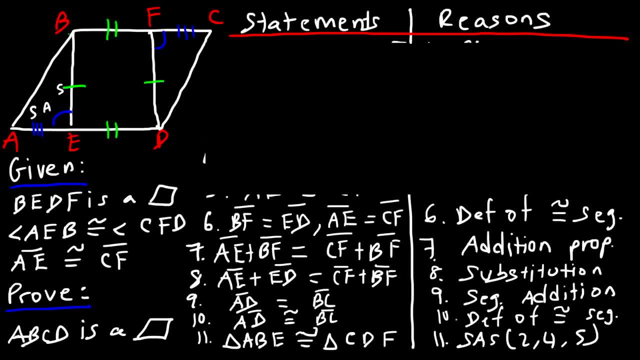 you can always rewind the video. so number 12: what can we say? since these two triangles are congruent, then all of their corresponding parts are congruent. so we can say that a, B and C, D are congruent. so a B is congruent to DC and 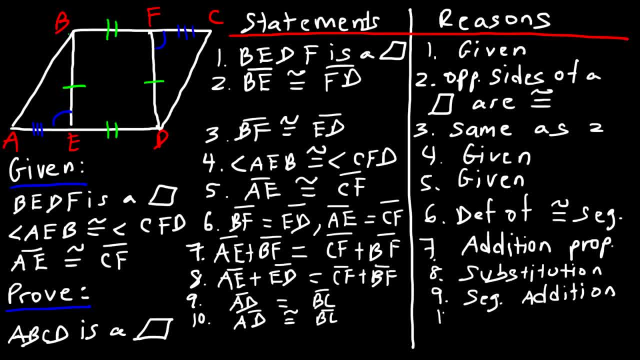 congruent to BC, and this is a definition of congruent segments. so now that we've shown that these two parts are congruent, we just need to show that these two are congruent each other and then we can prove that AB- CD is a parallelogram. so for number 11, notice that we can prove the triangles are. 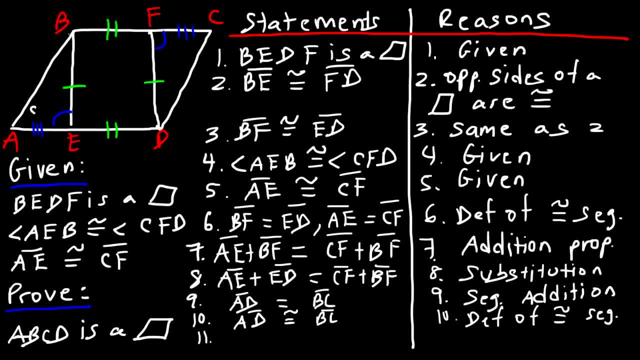 congruent using side angle side. so let's make this thing made that triangle a, B, e is congruent to triangle, to triangle side, angle side. So now let's make a statement that triangleiste is congruent to triangle, alte is congruent to trie. angle to distance plus cr is about bd and bd and bd equals ab to the right commute to side angle, so we can�. 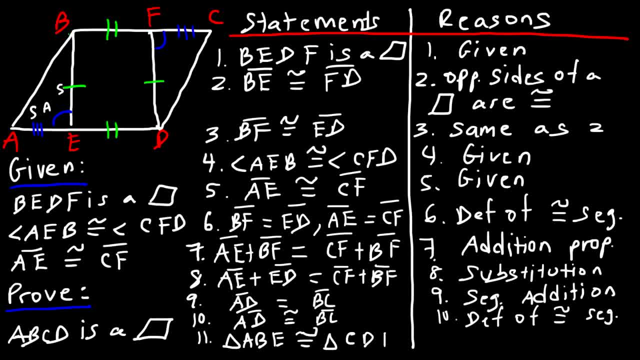 angle C, D, F. So A corresponds to C, B corresponds to D and E corresponds to F. So this is based on the SAS postulate and we've used AE, which is based on statements 5,, and AEB, which is based on statements 4,, and also BE is equal to FD, which is based 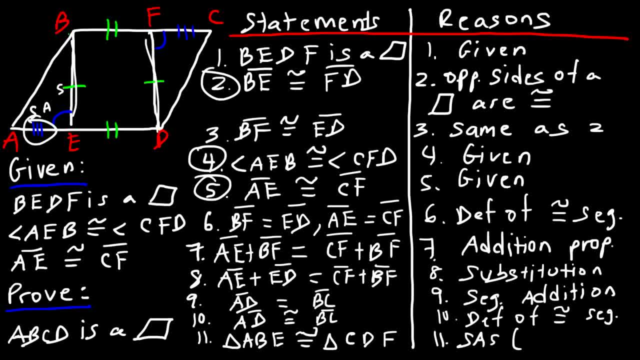 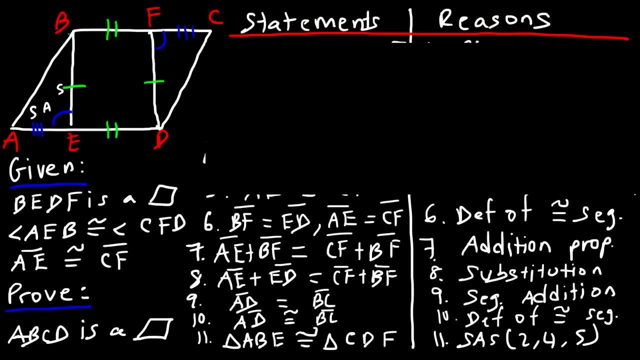 on 2.. So it's 2,, 4, and 5.. And now we have a problem. I am out of space, So I'm just going to get rid of this, Get rid of some stuff here. If you need it, you can always rewind the video. 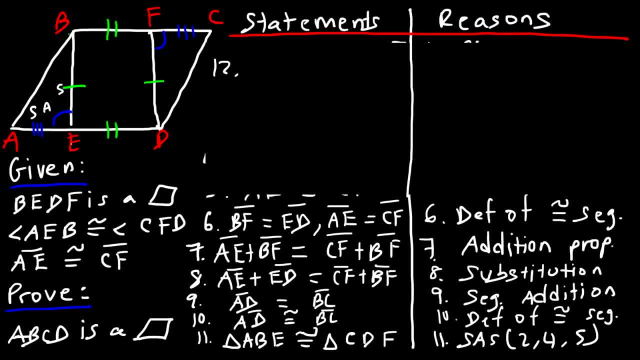 So number 12, what can we say? Since these two triangles are congruent, then all of their corresponding parts are congruent. So we can say that AB and CD are congruent. So AB is congruent to DC, And this is based on CPCTC.